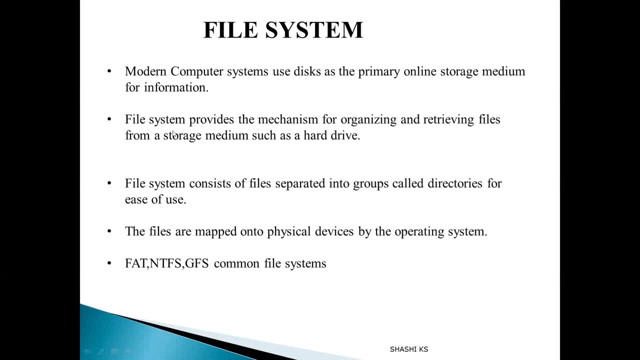 system is a concept which provides a mechanism for organization of the data which is stored in the secondary storage devices like a hard drive or a disk drive, etc. It also provides mechanisms for retrieving the files from the disk. Okay, so if you don't have a file system, then the files on the 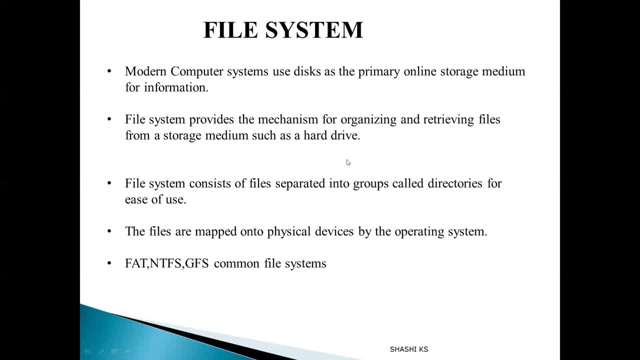 disk will not have a proper organization and retrieving all the files from the disk will also be not possible. It will be very difficult. Without the concept of file system we can't even have two files with the same names. So file system is the one which helps us to organize. 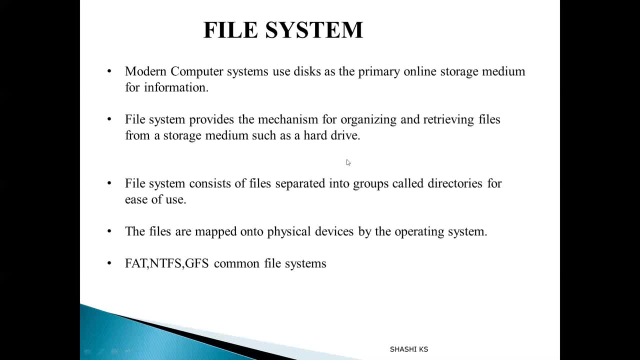 the files on the disk, as well as to retrieve or search for the files on the disk. Another important thing is: the different files in the file system are also grouped into categories called as directories. In Windows we will call this as folders, So files may be categorized. 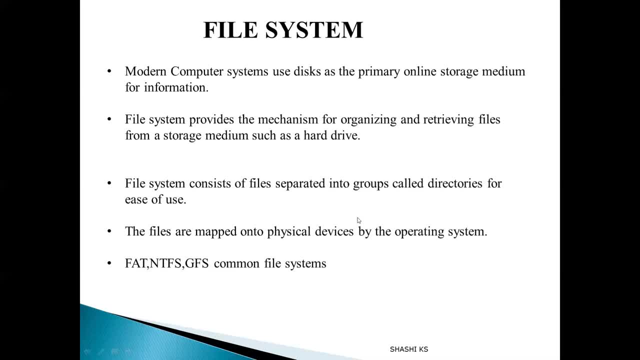 into directories for ease of use. And what is the role of the operating system here? We know that file is a logical storage unit. Whenever a user creates a file on a system, that is nothing but a logical storage unit. So the file is a logical storage unit. So 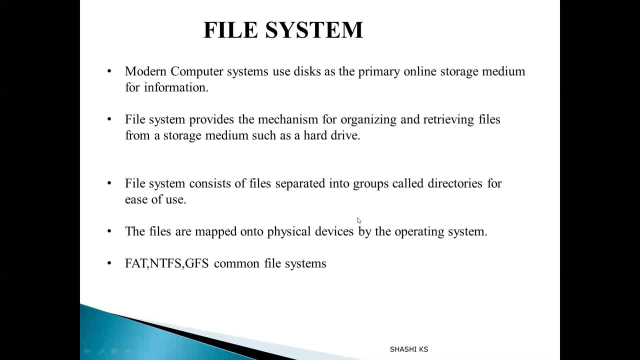 the file is a logical storage unit. Whenever a user creates a file on a system, that is nothing but a logical storage unit. So the file is a logical storage unit And the data which is stored or represented in the form of files is actually going to be stored on. 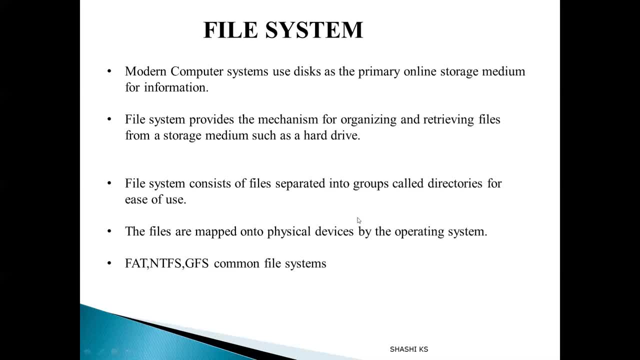 the physical devices which reside on the physical devices, which we call it a secondary memory. So this mapping between the logical storage unit of files is mapped onto the actual storage devices by the operating system. So that is the role of the operating system here. The 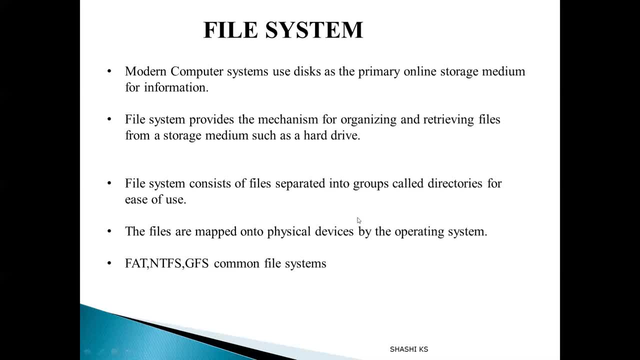 OS is responsible for mapping the logical files onto the real physical devices, which which we call it as secondary storage devices, And the most common file systems which we use in real time are the FAT file allocation table, which was used in the older versions of Windows. 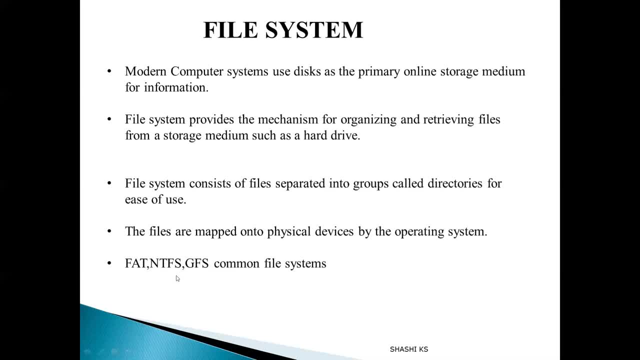 and then the NTFS file system, which is almost used in many versions of Windows, like Windows 7,, 8,, 10, Windows XP, Windows Vista, as well as it's also being used in Linux and BSD range of operating systems. 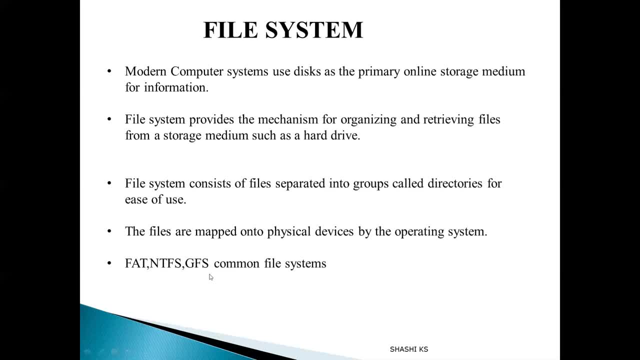 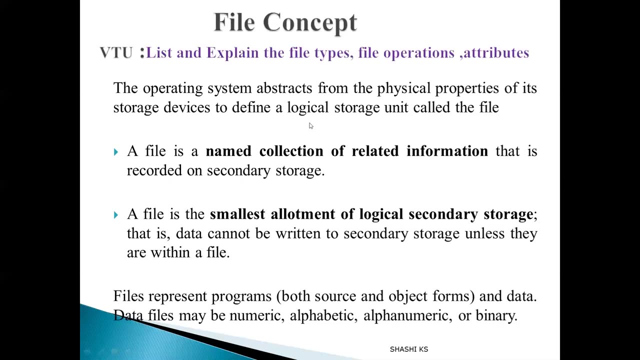 And then another common file system is the global file system, which is a shared disk file system which is being supported by Linux computer clusters. So these are all some common examples of file systems used by operating systems. So next, coming into our file concept, 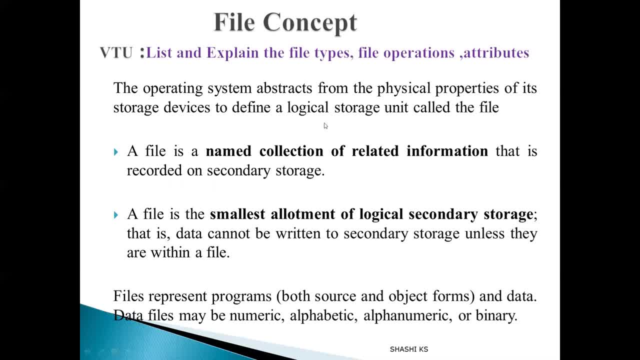 what is the meaning of a file? So a file is nothing, but it's. a file is a logical concept, It's a logical storage unit which is actually realized with the help of the physical properties of the storage devices present with the computer system. 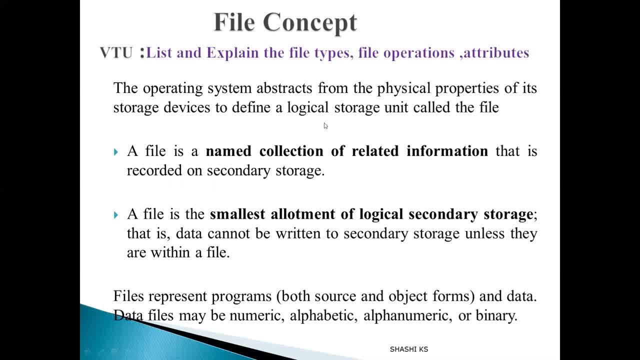 File is nothing but a logical unit and the data stored in the file is realized, or actually implemented, with the help of the storage which you get from the storage devices, with the help of the space available in the storage units. So the operating system abstracts the physical properties of the storage devices. 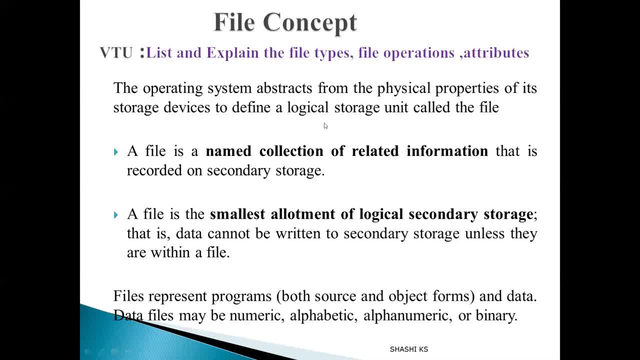 to define a logical storage unit called the file, And another definition is: this file can be called as a named collection of related information, which is defined by the file owner as well as it is being recorded on the secondary storage devices, So files can represent any type of data. 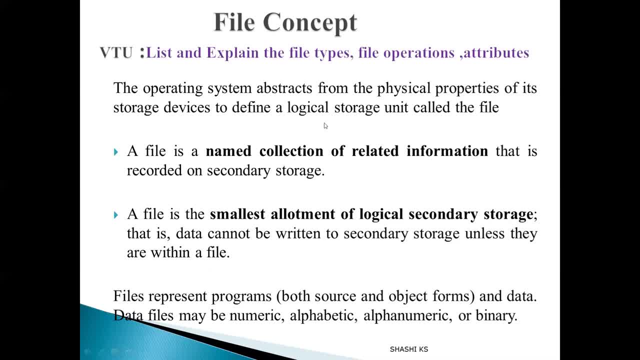 it can store programs. it can store any type of data. the data can be numeric data or alphanumeric data. it can store graphics, it can store sound recordings, it can store text, it can store numeric data, etc. So every file. 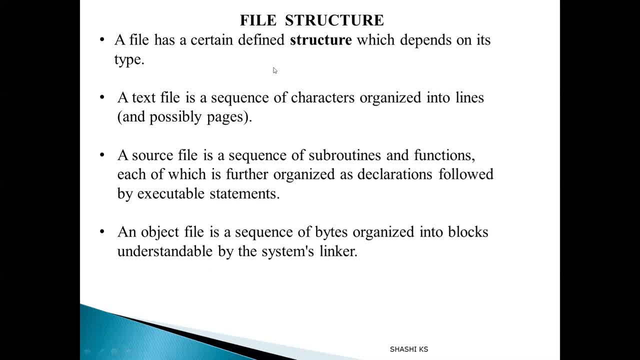 on. the file system has a certain structure, but all files don't follow the same structure. The structure of a file depends on the type of the file. So if you take a text file, the text file will be a sequence of characters which may be organized one line after the other. 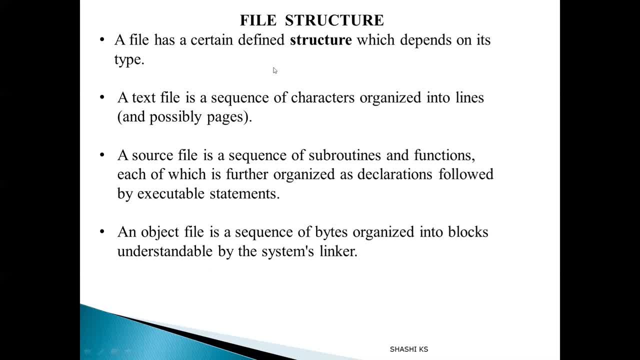 If you take a source program file, it may contain some header files, header file declarations. it may contain some declarations of variables. then it will be followed by some executable statements. It may also contain some sequences of function codes etc. So that is. 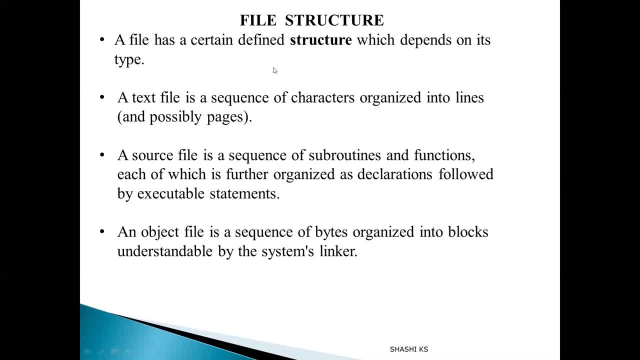 that is the structure for your source file. If it is an object file, we'll be having a sequence of bytes. bytes may be collected together to form blocks in such a way that it is understood by the program which is going to use it. 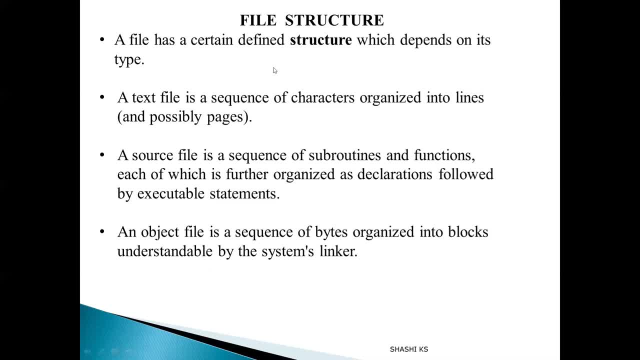 So here for our object file. the program which is going to use the object file is your linker. So object file will be in a format which can be understood by the linker. If you take an executable file, exe file, it will be a series of code sections so that it is possible for the loader to bring it into memory. 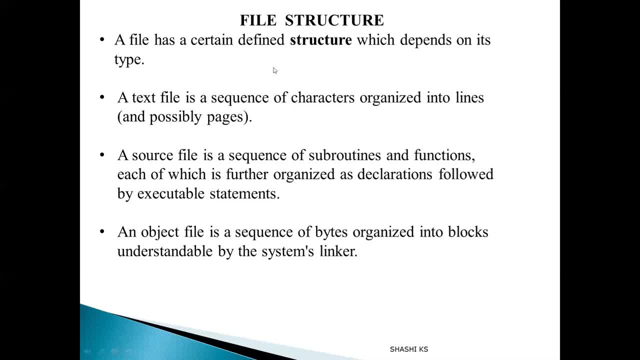 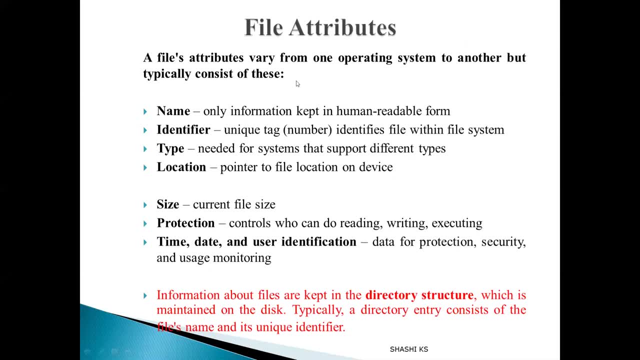 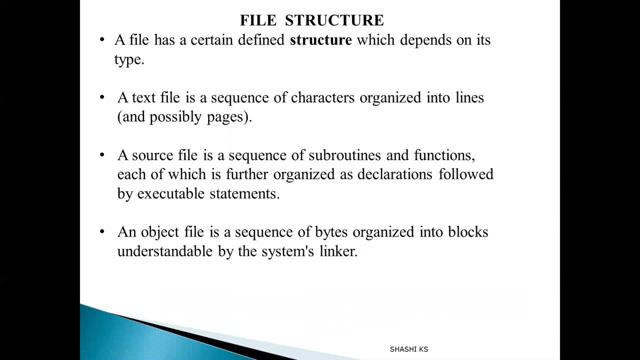 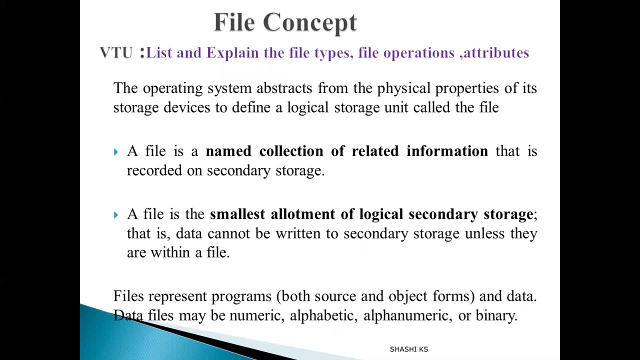 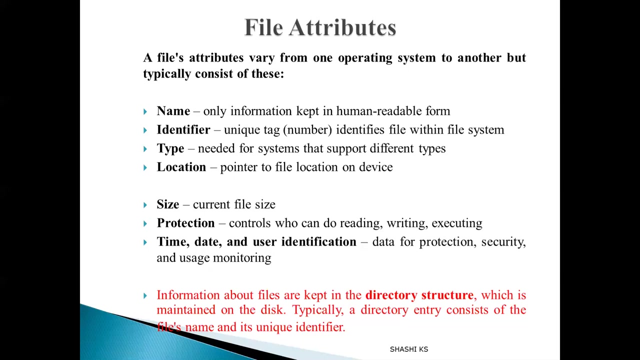 And execute. So every file has a certain structure which is dependent on the type of the file. So next is about the file attributes. So attributes, Yeah, Okay, So the attributes of the file. here we know that for to identify the file, will have an attribute called a file name. 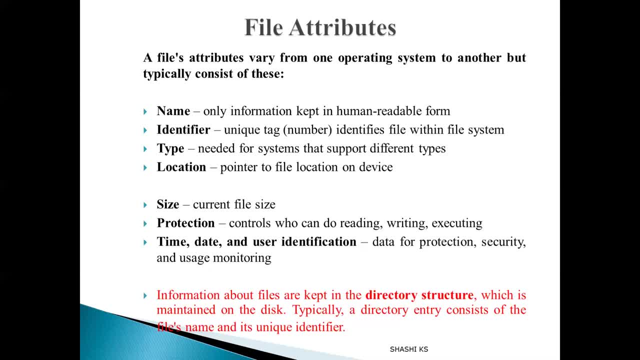 So all other attributes of the file may vary from one operating system to another. some of the common file attributes are listed here. So first attribute is the name- name of the file. we know that it is used to uniquely identify the file And most commonly 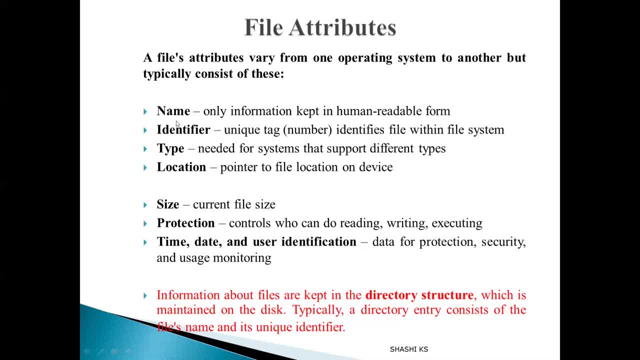 when we named the file, we gave the name for the file, followed by a dot, followed by a comma by the type of the file. this is used by the user to identify the file type. but no operating systems don't enforce that file type has to be mentioned by the user. so first attribute is name. name is: 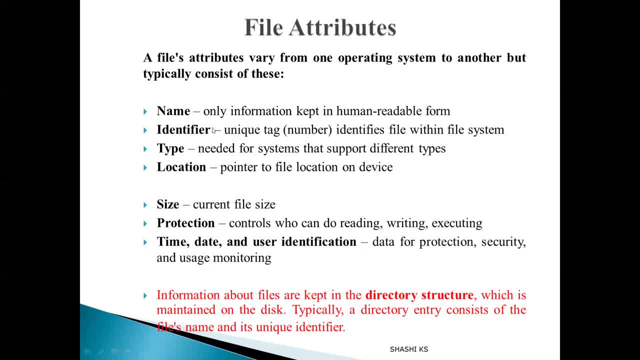 the only information which is kept in human readable form and this, this is used to identify the file. second is the identifier. now, this identifier will be a unique number which is used to identify the file within the files, but this identifier will not be in human readable form. it's it is in non-human readable form. the third one is the file type. so, if your system 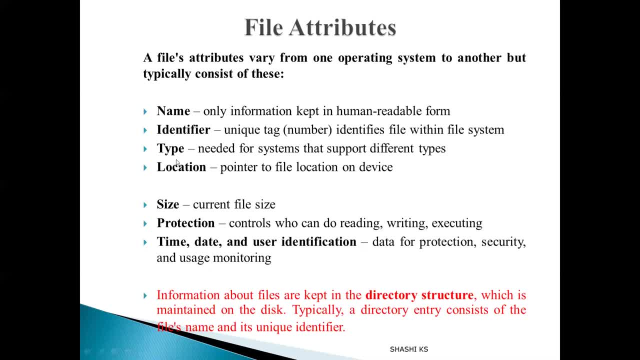 supports multiple different file types, then you have to mention the file type there. fourth one is the file location. now this is used to find the location of the file on the disk. fifth one is the size. size is used to represent what is the current size of the file. it might. 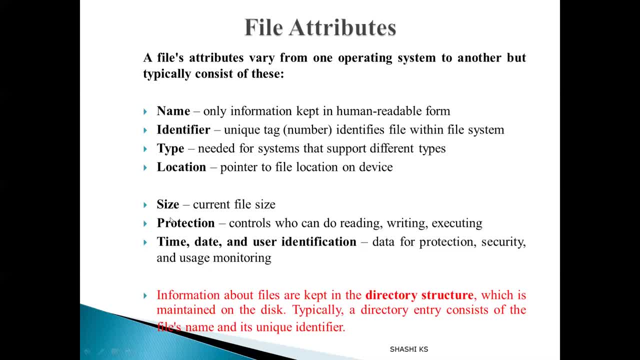 represented in bytes or words or blocks, or it may also. it may also contain information about what is the maximum allowed size for this particular file type. next attribute is file protection. this file protection attribute contains access, control information about which process is allowed to do the reading, read, write, execute operations on the file. next operation is the time, date and user. 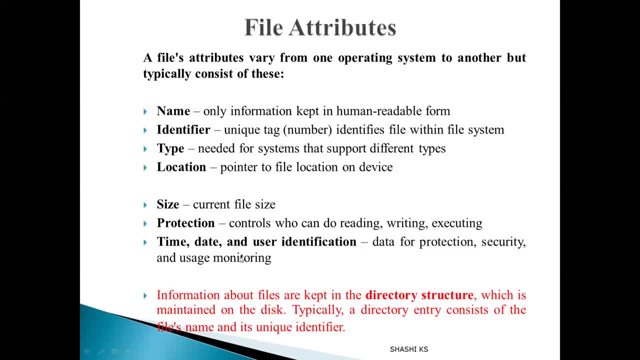 identification attribute, so this information is here. this attribute contains information about when the file was created, when it was last modified, when it was last used, etc. so we always uses this information for protection and security purposes, okay. so, apart from this, another important thing is you have something called as a directory structure. this is: 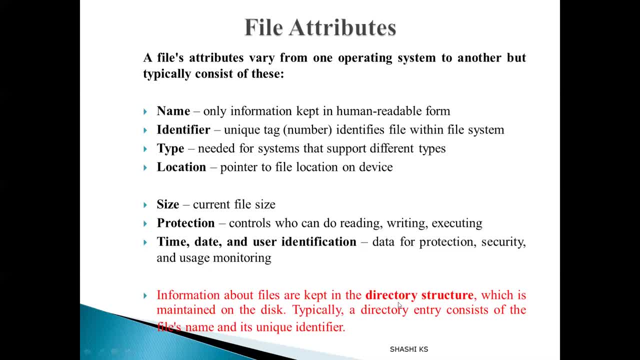 specifically used to contain information about all the files maintained on the disk. what information is maintained on the directory? directory structure is It is used to contain the file name and the file identifier. I told the first two file name and the file identifier Name will be in human readable form: identifier. 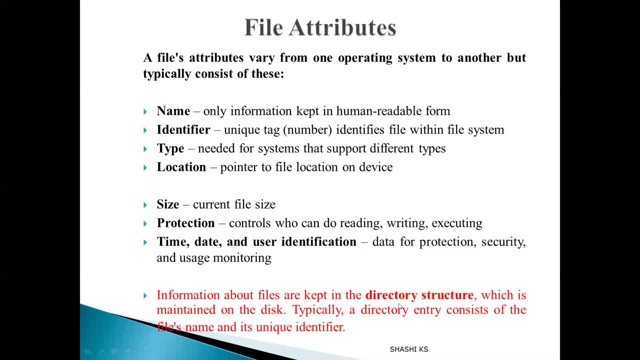 will not be in human readable form. Both these two are maintained by the directory entry and, apart from this, it may contain a pointer which points to the actual location of the file on the disk. And one more important thing is this directory structure will also reside. 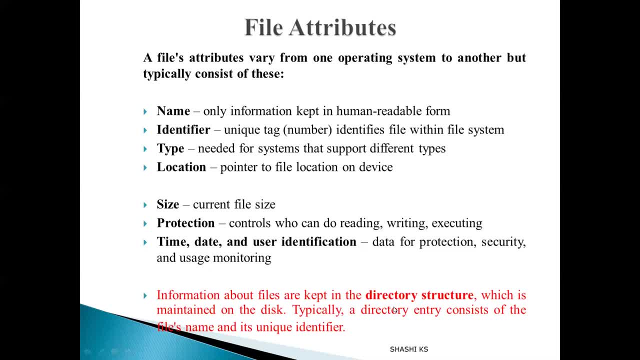 on the disk only. So sometimes what happens is if your file system stores too many number of files, it may take more than one kilobyte to record this information for each file. For each file, the information about the file may take up to one kilobyte of space, So this: 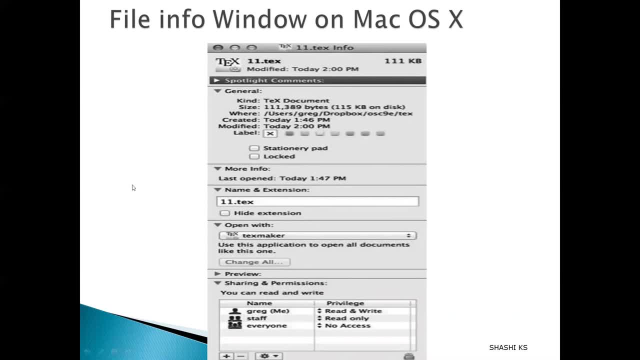 shows the file information window on macOS operating system. You can see that it stores information about the type of the file, size of the file in bytes, how much size on the disk, The location of the file when the file was created, at what time the file was created. 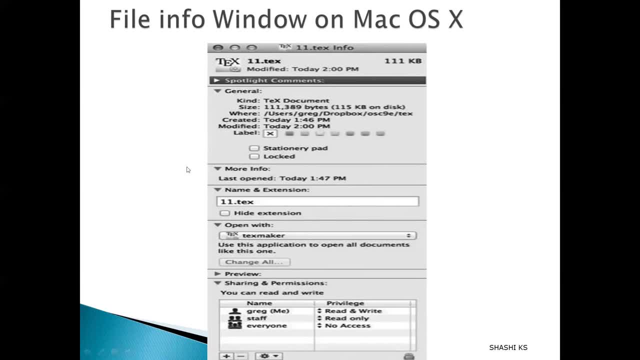 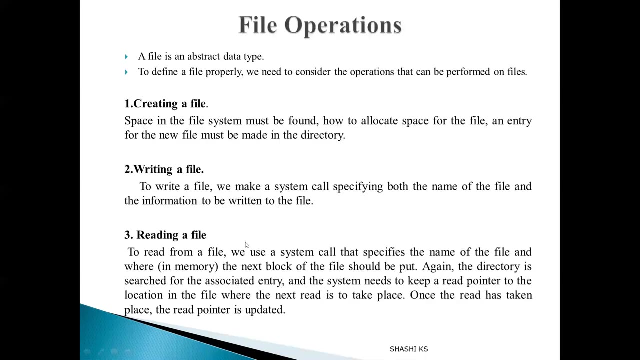 at what time the file was modified. All such informations are maintained in this file information window. Here you can see the file access permissions, also Who has what type of access, who doesn't have access. everything is being available. So next is about the file operations. So file. 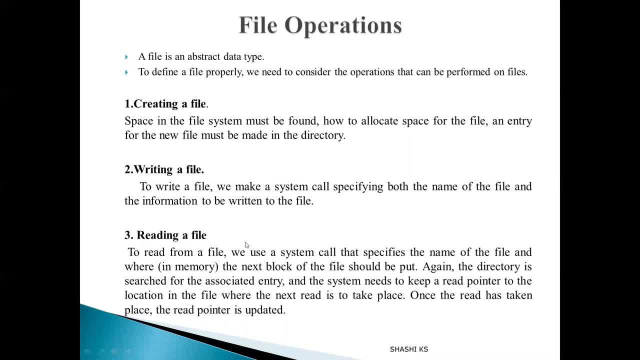 is just an abstract data type. So if you want to make use of the concept of file, you need to define the file. And to define the file properly, we need to define the operations which can be performed on the files. So there are six different types of operations which 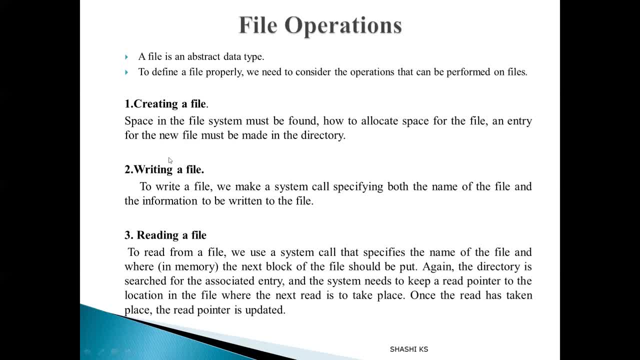 can be performed on the file, And the OS provides various system calls to implement these operations. For example, for open, you have the open system. called. for read, you have the read system. called. for write, you have the write system called, etc. So first one is the creation. 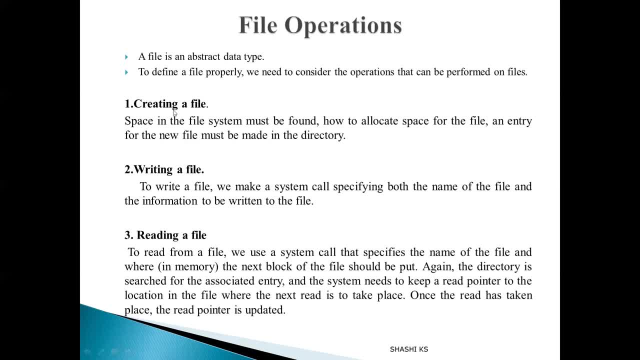 of the file. So to create a file, first space has to be available, found in the file system for the file, And then an entry has to be created for the for the file in the directory. Okay, so once this is done, a file is created and then an entry for the file is made in the directory. 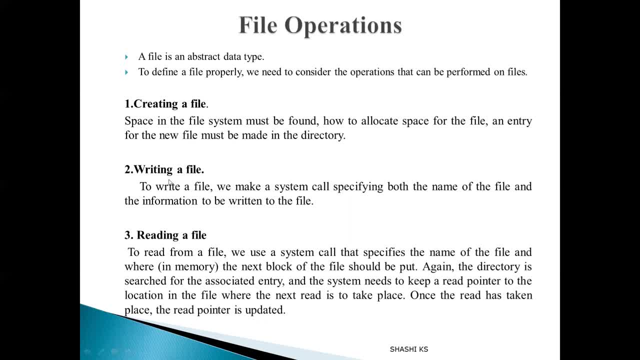 The second file operation is writing a file. So to write to a file the user will make use of the write system called specifying the name of the file and what information has to be written to the file, And then the system will search the directory to find the 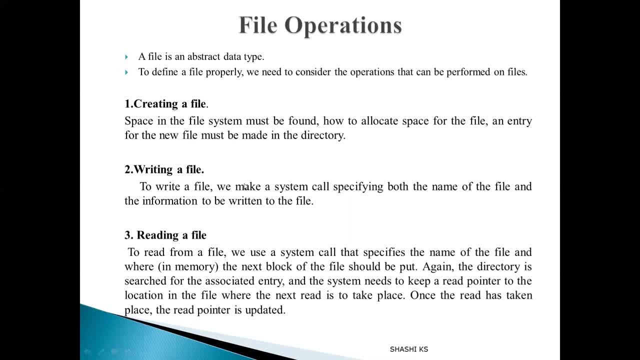 log files location. The second file operation is the read system, called the read system. So to read the file, the user has to be able to specify the location where the next write has to take place, And after the write operation is completed, the write pointer will be updated. So this is. 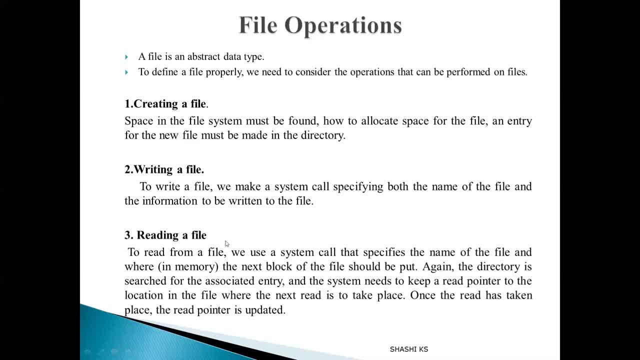 how write operation takes place. Third, one is reading a file. again, for reading the file we use a read system called, where we have to specify the name of the file and where that the block of the file has to be if you're reading the contents of the file to the memory. 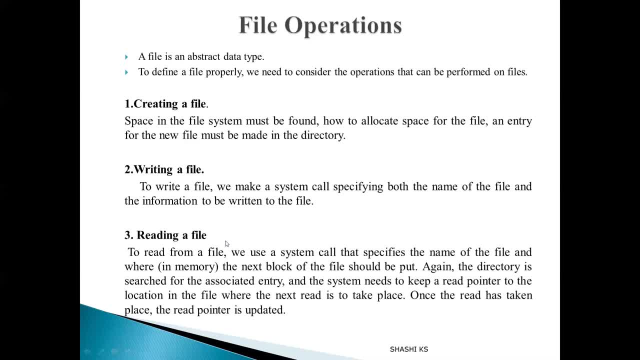 so where it has to be put into memory that information can also be mentioned. So again, So again. the directory entry will be searched for the corresponding file and the system will make use of a read pointer which will contain the location where the next read has to take place. 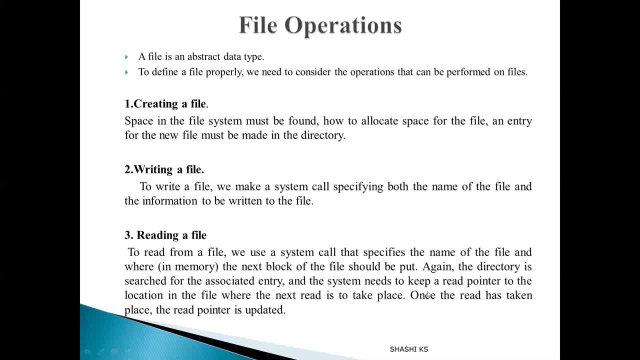 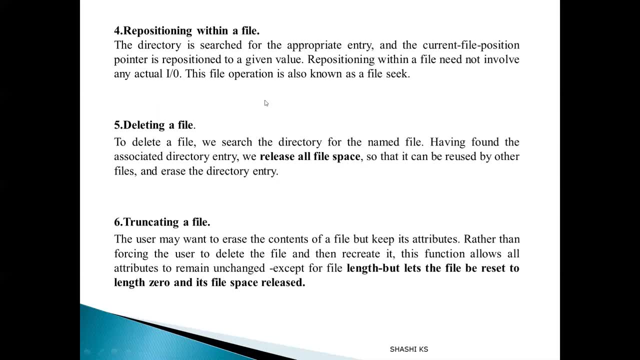 In case read is taking place record by record, then read pointer will be updated after every read operation. The fourth operation is repositioning a file. Here no input output is actually carried out, Simply the file pointer will be repositioned. The file pointer location will be changed to the location which is specified in the system call. 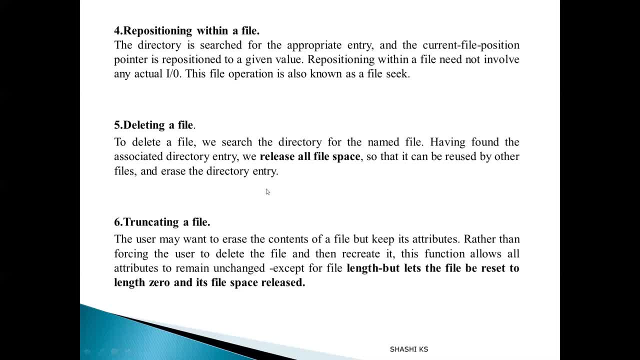 Fifth one is deleting a file. So to delete a file, first of all the OS has to search the directory for that particular file And then, once the file entry is found in the directory, then all the memory which has been allocated to the file, all the space which is allocated to the file on the disk, everything has to be released. 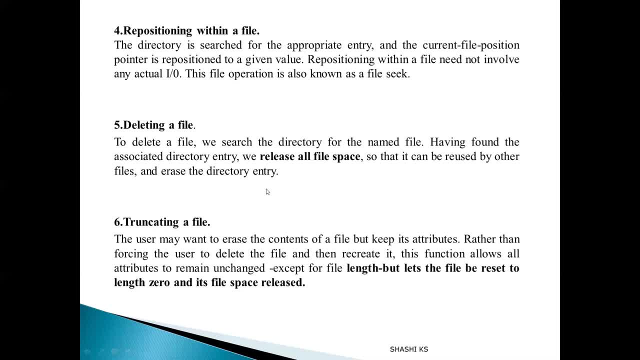 And then the entry file has to be deleted And for that file in the directory also will be deleted. The last file operation is truncating a file. So if you want to maintain the file and its attributes but you don't want to maintain the contents of the file, then you will make use of the truncation operation. 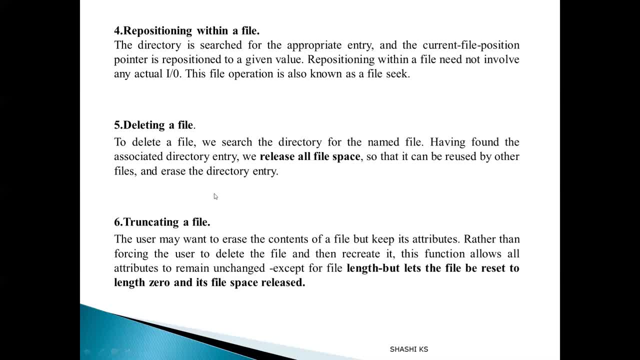 So here the file will be reset to length 0.. All the space allocated to the file will be released, But the file will be existing with its attributes. So that is about the different types of file operations. So there are six different types of file operations. 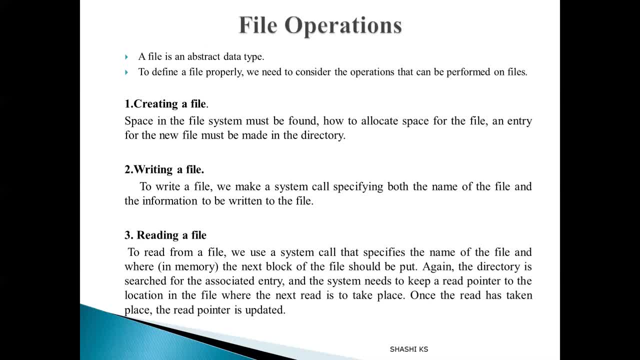 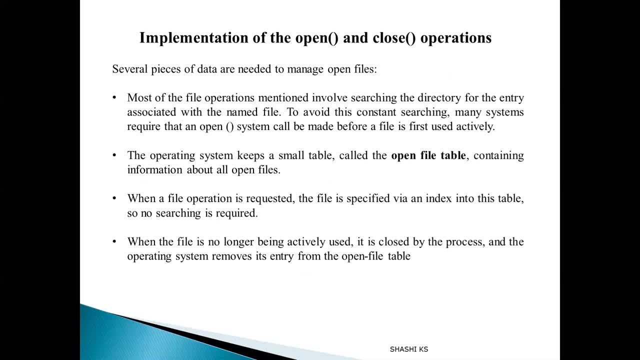 Namely file creation, file deletion, reading, writing, repositioning and truncating a file. So next is about the implementation of the open and the close operations. When your system supports multiple processes to share the files, then the implementation of open and close operation requires some data structures. 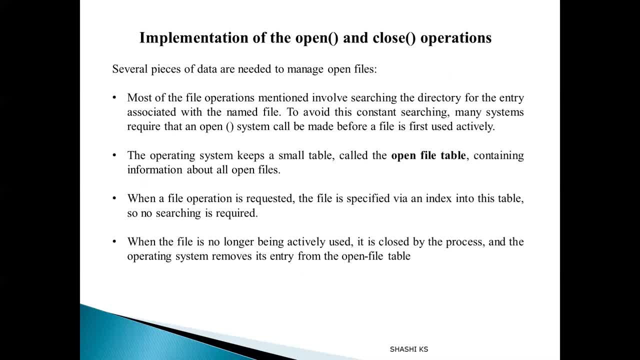 Because every time, whenever a process wants to open a file, searching the directory entry will be a very tedious task. So in order to avoid frequent searching of the directory entry, OAS maintains a small data structure called as the open file table. Now this open file table contains information about all the open files in the system. 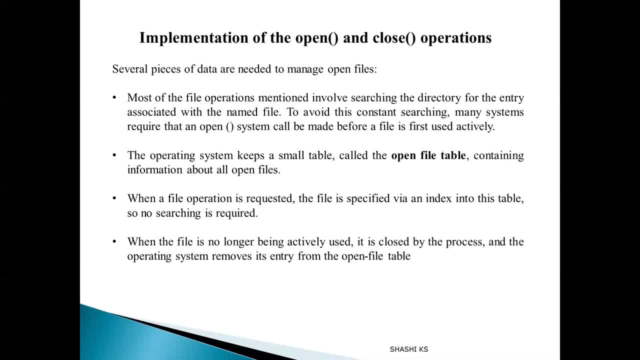 So whenever a file has to be searched, whenever a file operation has been requested, then through the index of this open file table, the file will be searched for, so that there is no requirement for you to search in the directory entry for the file. 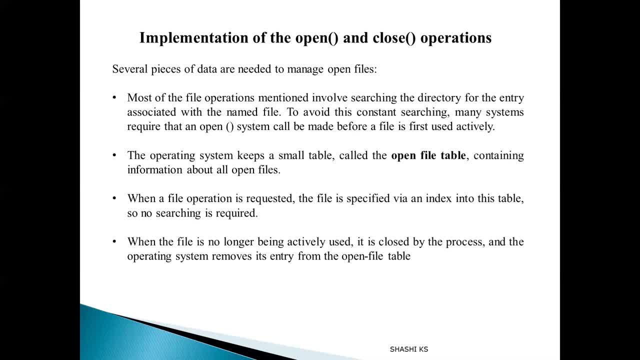 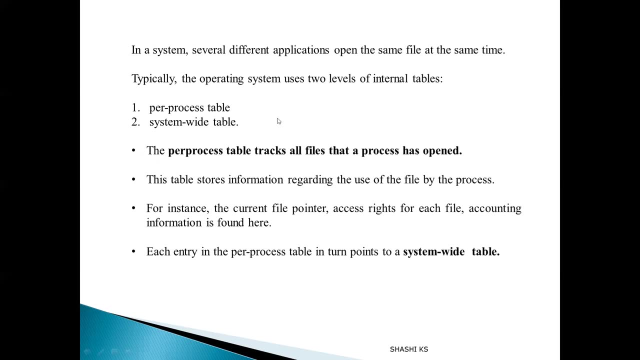 Whenever a file is closed by the process and the file is no longer used, that entry for the file will be removed from the open file table. Two more data structures which has been used by the operating system is per process table and the system-wide table. 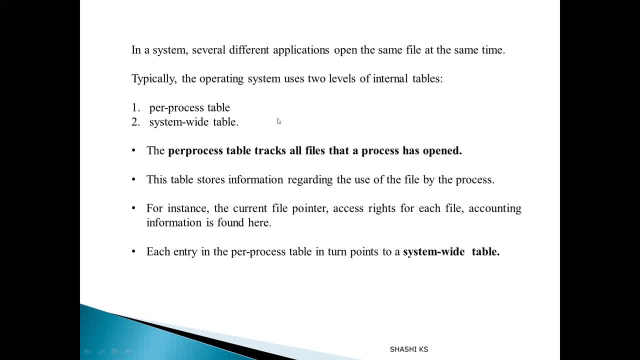 Now this per process table tracks a list of all the files which has been opened by a process. Each per process table contains a pointer to the system-wide table And this system-wide table. what it will do is, whenever a file is opened by a process, an entry for the file is made in the open file table. 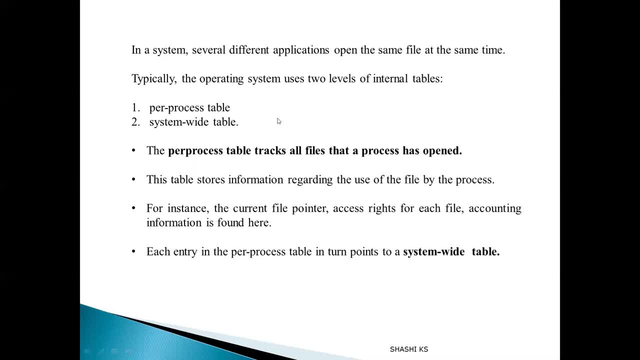 Remember that open file table is the one which I told you previously. An entry for the file is made in the open file table, which in turn will point to an entry in the system-wide table. If later, let's say, another process opens the file, then an entry, another new entry will be made in the open file table. 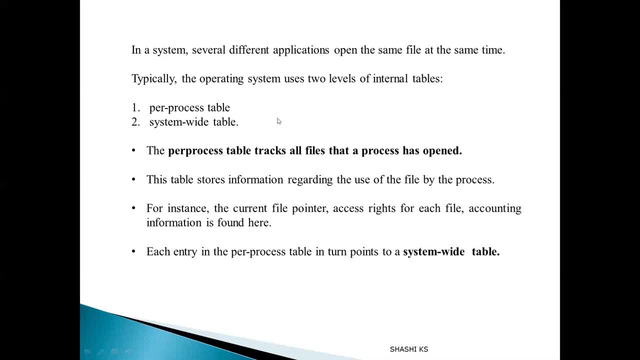 But it will again point to the same entry in the system-wide table. So in this way system-wide table can keep track of what are all the processes which are working on any particular file. So it maintains information about all the files in the system. 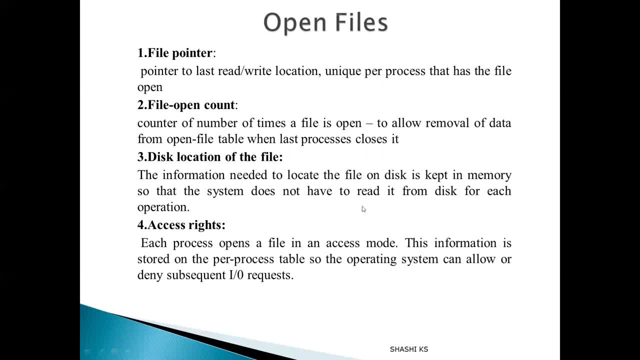 So all the files which are open in the system, they will have the following four information associated with them. So this piece of information will be maintained for all the open files. First one is file pointer. File pointer is used for finding the next read location or the next write location. 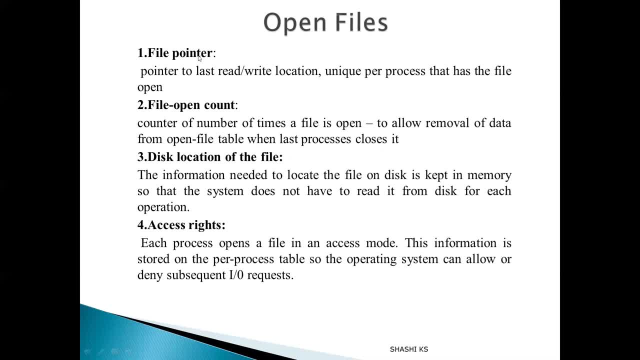 Whenever a read or write operation is performed, the file pointer is updated to point to the next record or to the next location inside the file where the next read or write operation has to take place. Next is file open count. It keeps a list of all the processes which has opened the file. 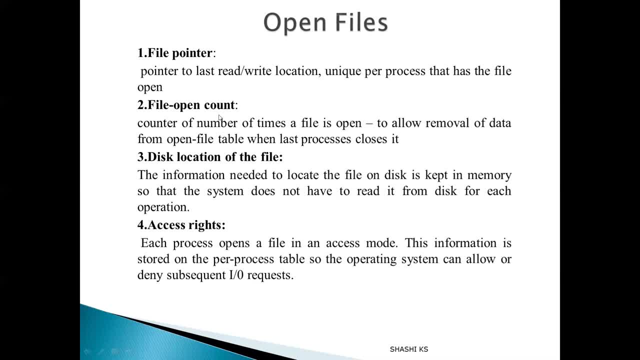 So when file open count becomes zero it means no process is currently used. So the entry for the file will be removed from the open file table. Third one is disk location of the file. So this specifies the location of the file on the disk. 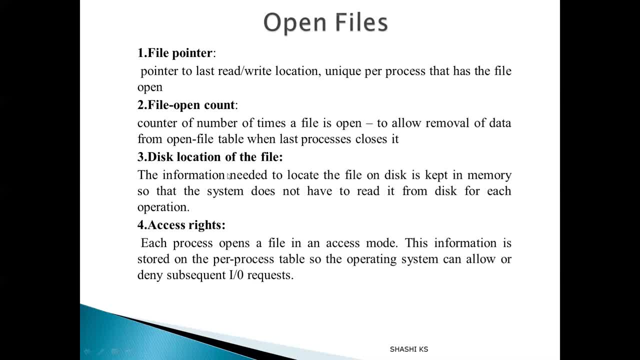 This is useful if you want to bring the file from the disk to memory. Then it facilitates easier retrieval. Fourth one is access rights. So every process is allowed to open a file in a particular access mode. So this access rights information contains contains what type of access rights protection that particular process has. 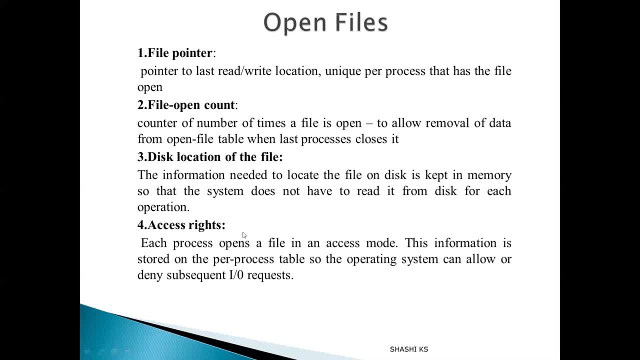 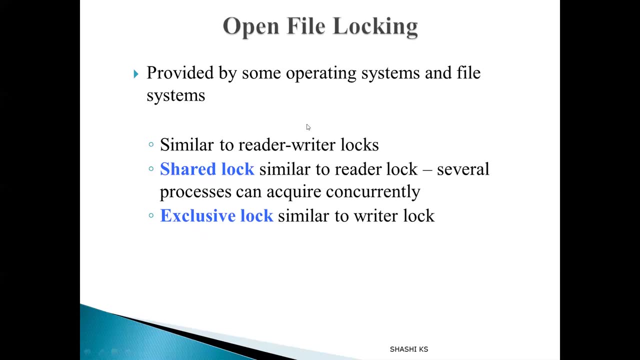 So that if the process tries to use that file in some other mode, then the operating system can allow or deny it based on the access rights for that particular file for the process. So some operating systems also provide facilities for file locking. Whenever a file is opened, then the process can get some locks, called as shared locks or exclusive locks. 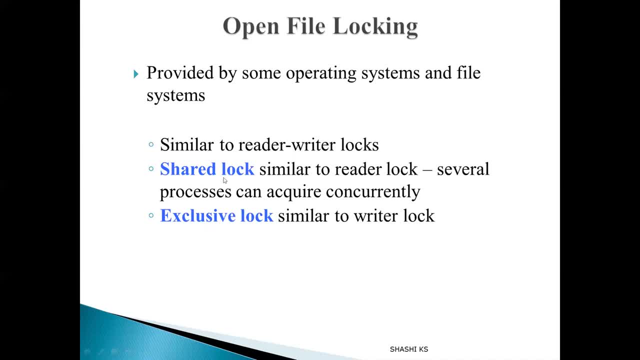 Shared locks are nothing but Previously we learnt about reader-writer problem, So similar to that: if multiple processes want to read a file simultaneously, they can get a shared lock. If some process wants to write to a file, then it can get an exclusive lock and write to the file. 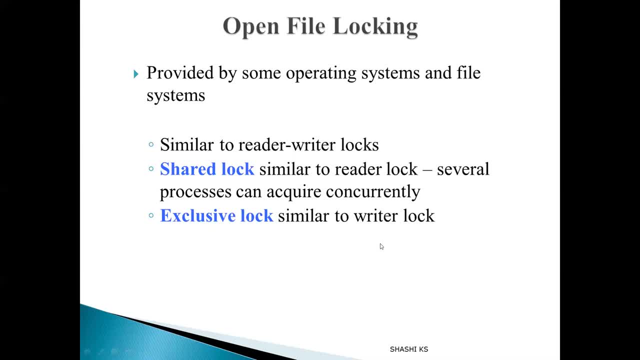 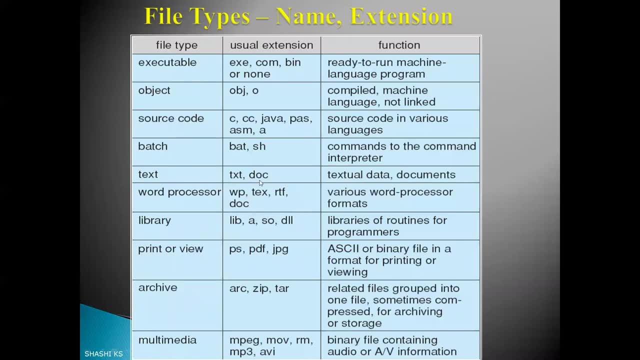 So this facility is provided by some types of operating systems. So that is all about the different types of file operations. We saw that there are six types of file operations. The next is about the different types of file types. So every file is specified or saved with a file name, followed by a dot, followed by an extension. 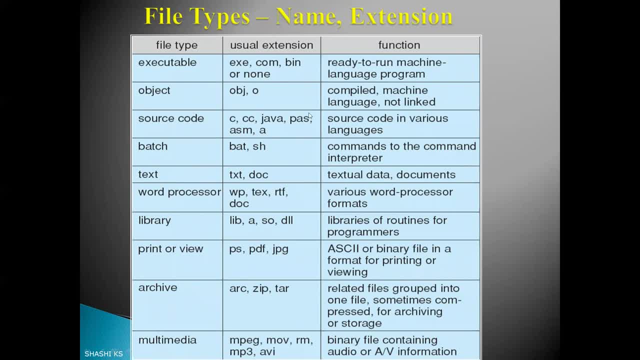 And that extension usually specifies the type of the file. These are some commonly used file types. First is executable files. File types can be categorized into these categories, So executable files, Executable files are ready to run files. They can be. We can load an executable file into memory to get the output for our code. 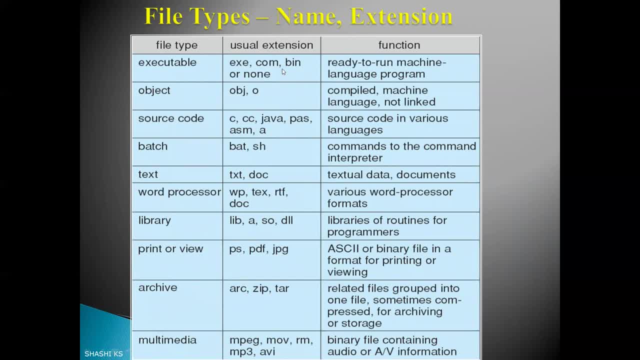 So they usually have these extensions, namely exe, bin, com, etc. The second type of file is object files. They usually have the extension obj or o. This means that these types of files will contain machine language code, or also called as object code. 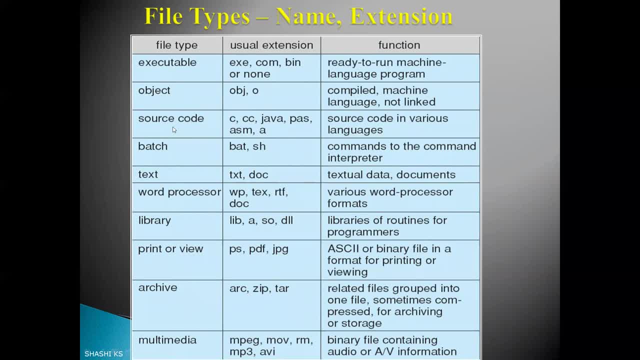 But they will not be linked. Third type of files is the source code files. These are nothing but the files which are written in some particular programming language. For example, your C code may have the extension c. Your Java file might have the extension java. 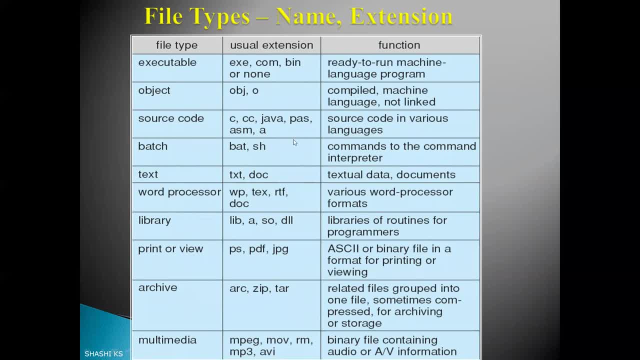 Your Pascal program may contain the extension pas. Your assembler program may contain the extension asm. Your library file may contain the extension a, etc. Similarly, command interpreter programs will have the extension bat or sh. They are called batch files. 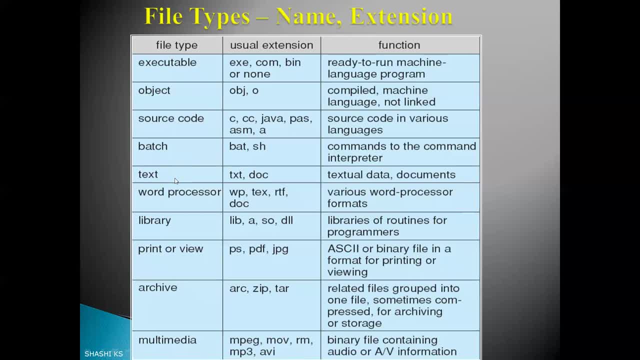 Text files may have the extension sh, Like txt, doc. Word processor files may have the extension wp, txt, rtf, etc. Library files may have the extension lib a, so, dll, etc. 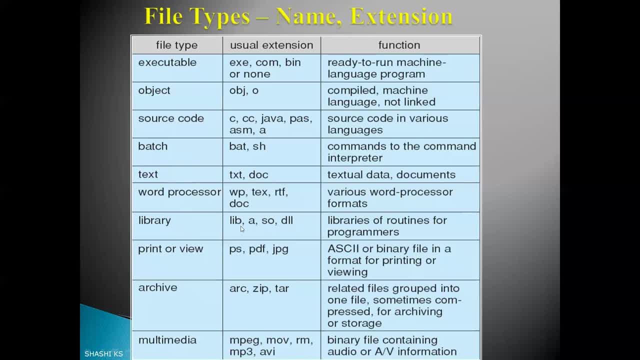 So here a stands for archived library files And so stands for shared object files. So the difference between these two is: a archived library files makes use of stack files. a archived library files makes use of stack files. 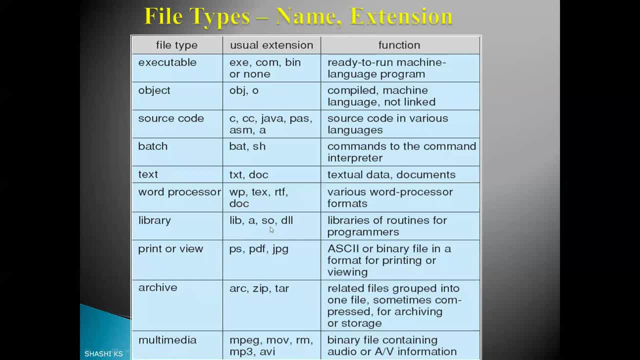 p. archived library files makes use of static linking And ps, so shared object files makes use of dynamic linking And then Printing or viewing file types is You have ps, which stands for post script, pdf and jpg. 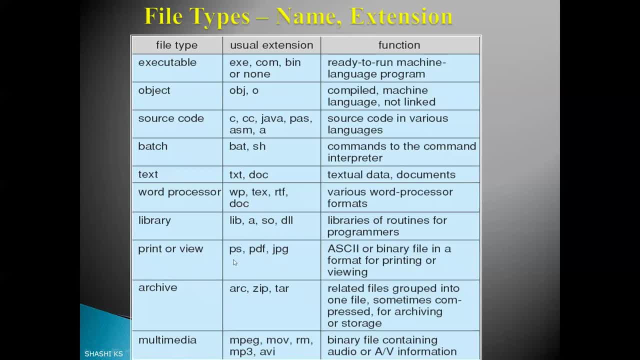 And so here, ps postscript files are commonly used printing file formats which are used in the publishing industry. We will also have many archive files. commonly we would have encountered these type of files. We use this zip or tar files for. 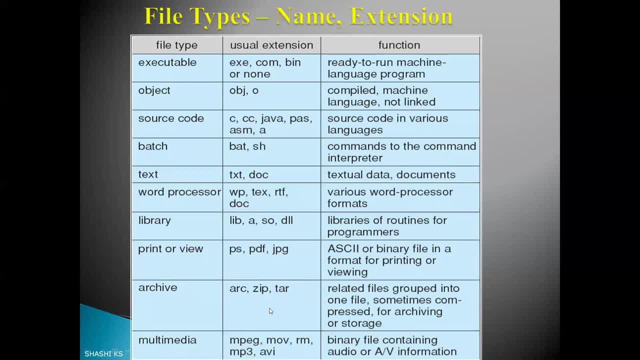 compressing the files and sending them over the network, etc. And then we have a large range of multimedia file types. Some of them are listed here: mpeg, mov, mp3, mp4.. And then we have flv files, av files, rm- rm stands for real media, So this is used. 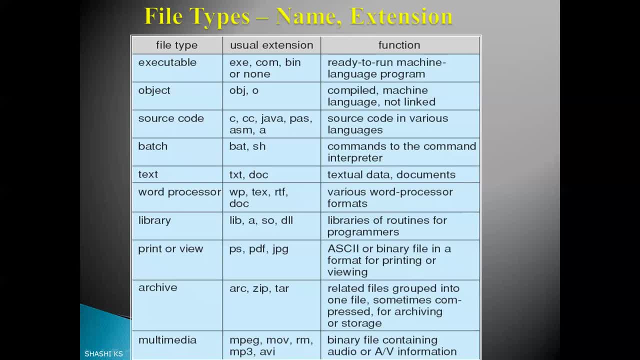 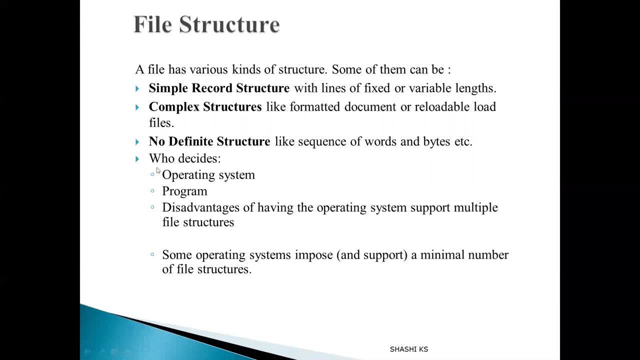 for streaming the content over the internet. So these are some common examples of file types and their extensions. Next is about file structure. A file can have three types of structures and operating systems. most of the operating systems support only minimal number of file structures. Why they support only minimal number of file structures is: 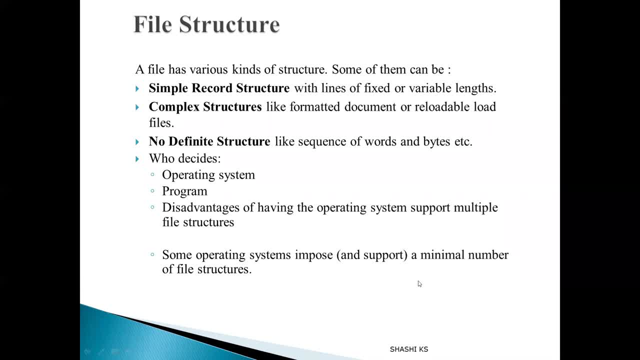 if an operating system supports more number of file structures. let's say, if an OS supports five types of files, then it supports five types of files. So if an OS supports five types of file structures, then it has to incorporate the code for supporting all these. 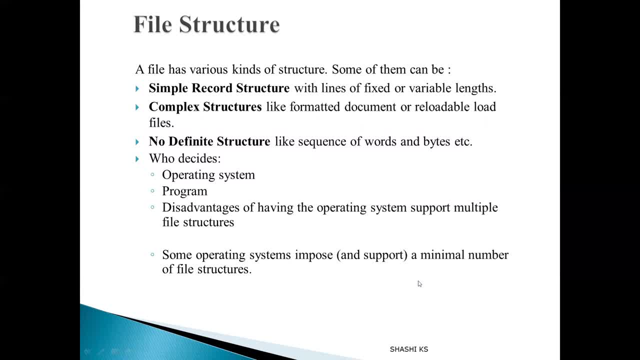 file structures And in that way the size of the operating system becomes large. So in order to avoid that, most of the operating systems support only minimal number of file structures- For example in Unix or MS-DOS operating system the file is supposed to- 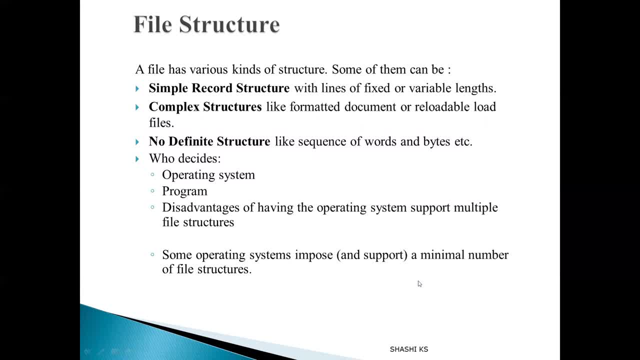 be a sequence of eight bit bytes. No other interpretation of the bits is made by the operating system. So there are three types of file structures. One is it cannot. it may not have any definite structure. So in that case that OS will consider the file as a 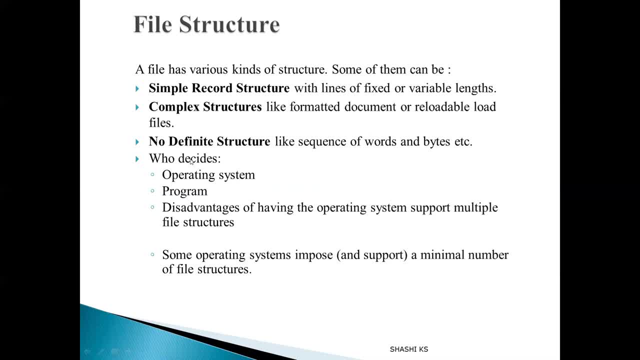 sequence of words or a sequence of bytes or something like that. The other one is simple record structure. We can define a file to be some fixed number of lines of some fixed length or varying length. Third one is complex structure. Complex structure means that if 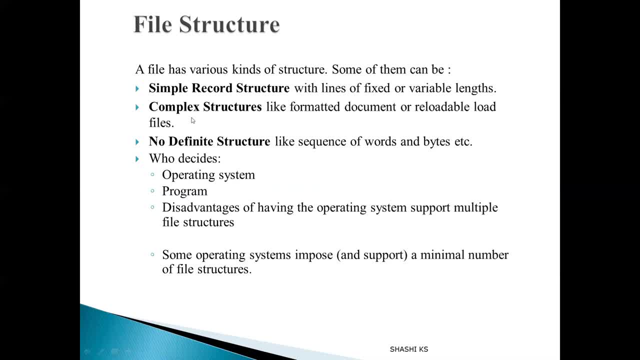 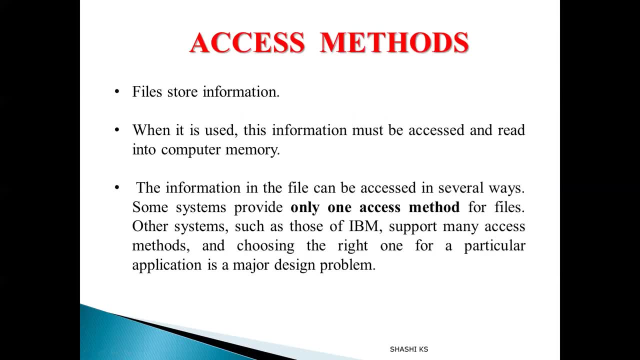 your file is a formatted document which has to follow a fixed format, or if it is a reloadable load files. all these types of files will come under complex structure. So if you have a file that is not a file, you can call it a file structure. So that is all about the 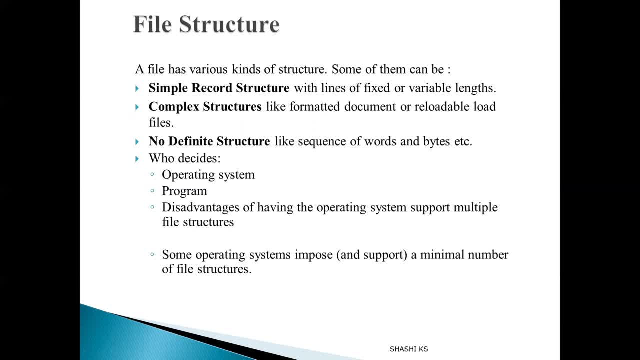 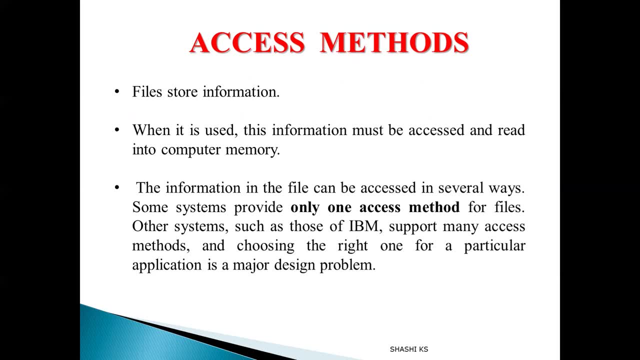 different types of file structures. With this, the concept of file concept is over. The next is about the different types of file access methods. So we all know that files store a lot of information. We store- OS stores information in ranges of millions or billions of bytes. 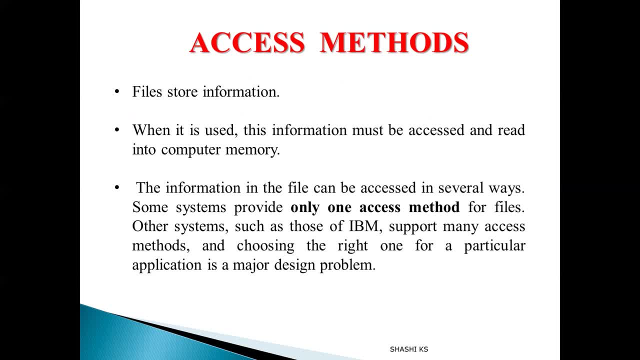 bits of information. So there should be some way for the OS to access this information and read it into the computer. So that is all about the different types of file structures. So for that there are two types of access methods commonly used. One is sequential access. 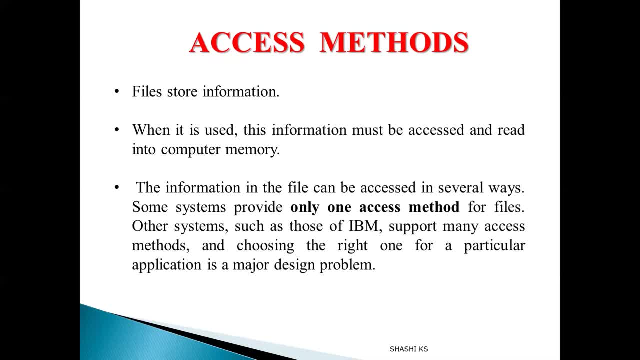 method and the other one is direct access method. So some operating systems provide support for only one type of access method. Some OS provide support for more than one access method. In that case it is the responsibility of the application to choose which access method. 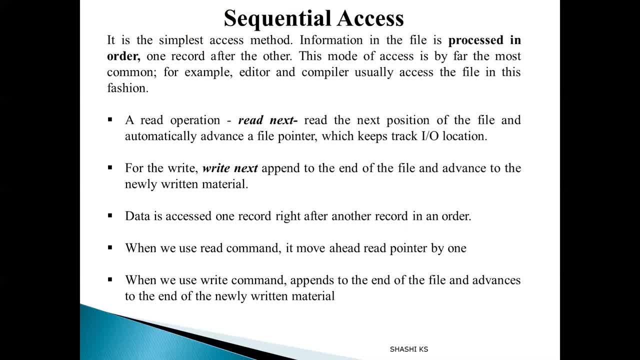 to use. So first type of access method is called us sequential access method. As the name suggests, the information stored in the file will be accessed or processed in sequential order. Sequential order means one record after the other, For example editors or compilers. 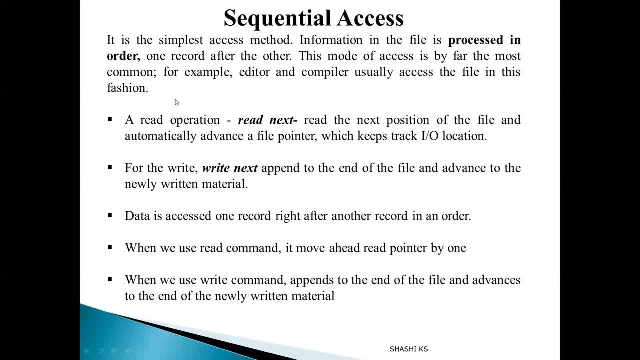 make use of this sequential access method. If you want to access record number 15, you must start from record number 1, move to 2, 3,, 4, 5, 6 and so on and reach record number 15.. So here there are two types of operations. The first is the stackable operation, The stackable operation is when the stackable transaction is performed. This is the type of operation that we use often. Let's see how it works. So the stackable operation is when we go to the stackable transaction and access. the stored records are stored, and then when we go to the 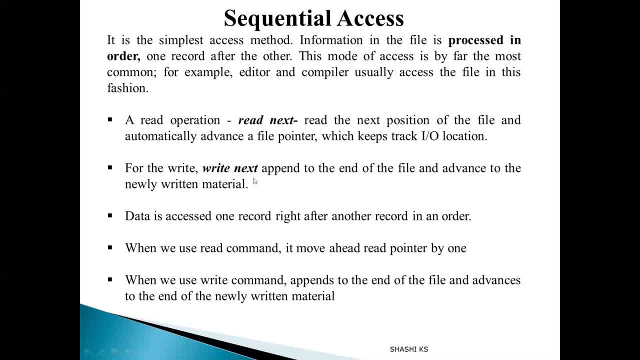 read operation is given by read next and write operation is given by write next, where you would be having a file pointer. So, file pointer, whichever position the file pointer is pointing to, read operation will read that particular record and then advances the file pointer to the next record. 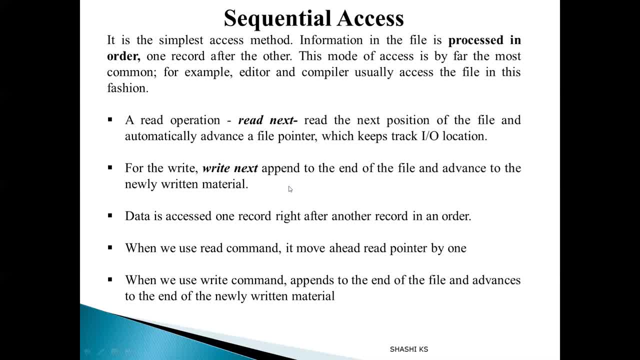 Similarly for the write operation. the write operation will check the position of the write pointer. It will write the contents of the file, new information and then, finally, it will advance the write pointer to the end of the newly written file. But one thing to remember is: 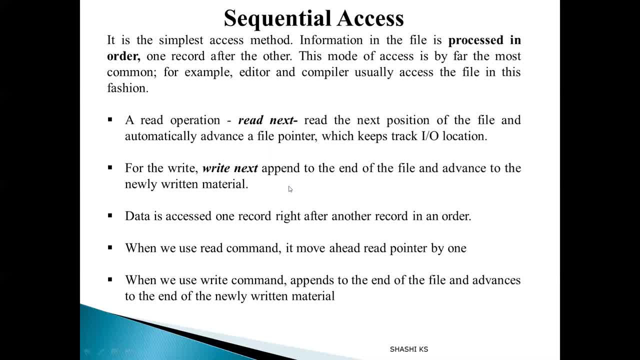 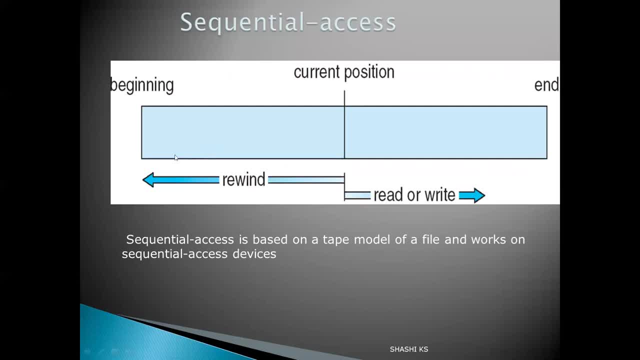 always the read pointer or the write pointer is moved ahead one by one, one record after another. So this is a diagram which shows a concept of sequential access. You can see that the rewinding is also possible where a program may be able to skip backward. 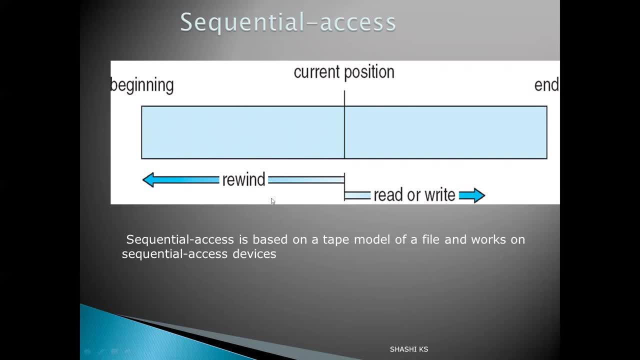 for some n integers, and it also shows the beginning and the end of the file. So this resembles a tape model of a file, where the records of the file can be accessed in order, one after the other. One record after the other only can be accessed. 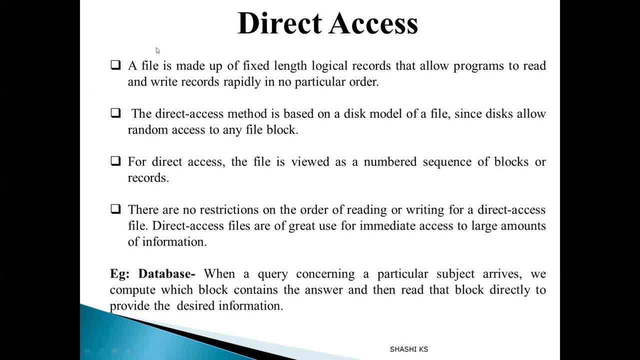 Second type of access is called as direct access. So here in direct access we assume that file is made up of fixed length logical records, but then the records can be accessed randomly in any order. So there is no particular order which you have to follow to read or write the record. 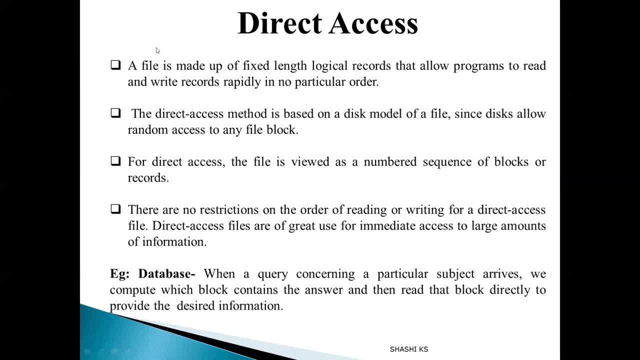 but then they can be accessed randomly. So direct access is also called as relative access and we can say that it resembles a disk model of a file, because if you imagine the disk model, any record can be randomly accessed from any location. So that is this: direct access or relative access. 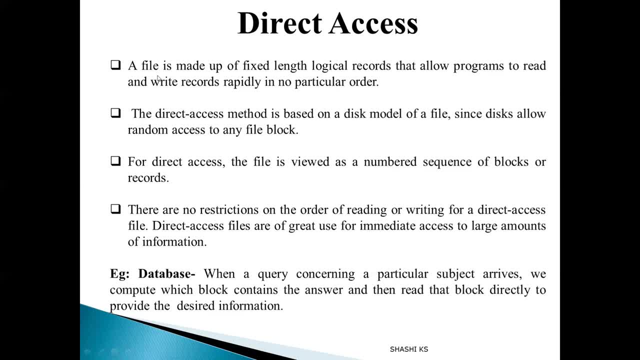 So here this is being followed by databases. We saw that sequential access is used by compilers or editors, but direct access is used by database. suppose we present the, suppose a query arrives to the operating system, then what the database will do is it will compute the particular block where that 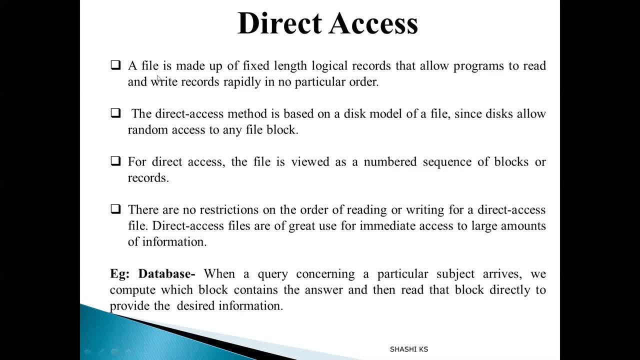 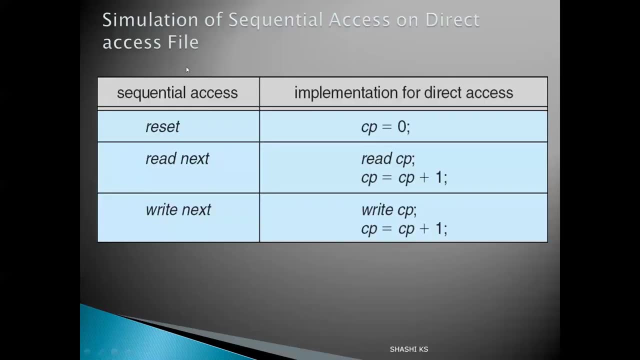 particular information is available and directly it will try to access the information in that block. okay, so this is useful when you have to access large amounts of information because you don't have a restriction that you have to follow or access the records one after the other. so if you want to simulate sequential access on direct access, we know the 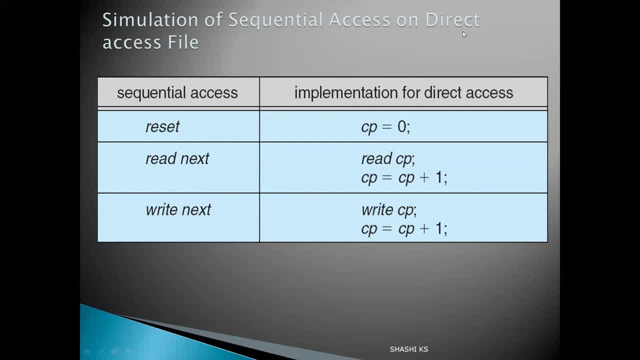 sequential access is ordered access. direct access is random access. so if you want to do this ordered access on the random access, the implementation may look like this. so reset to the beginning of the file can be done by you setting the current pointer to zero. read next operation can be implemented like this: 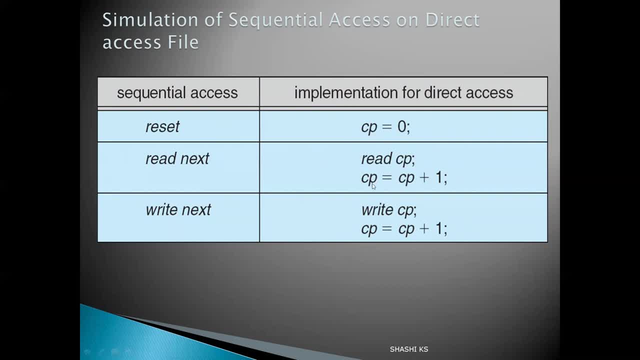 we can read the current position of the current pointer and then current. after doing the reading operation, the value of the current pointer can be implemented by one right. next can be implemented like this: we can. we can write to the right. we can first get the current position of the current pointer, write the contents of the file and then 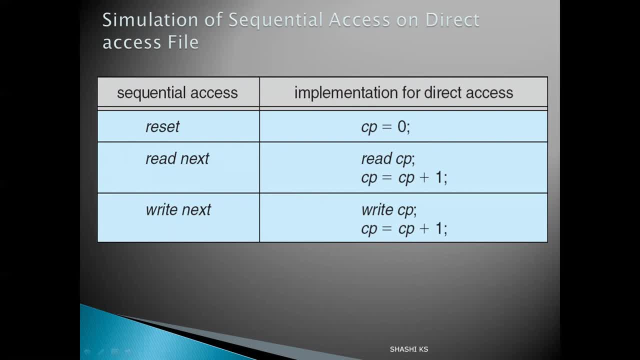 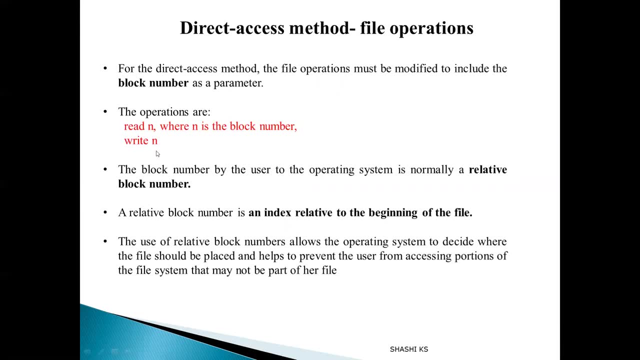 the value of the current pointer will be incremented by one, so file operations in direct access method will look like read n and write n. we just saw that in sequential access it was read next and write next. we will be able to only sequentially access one record after the other. 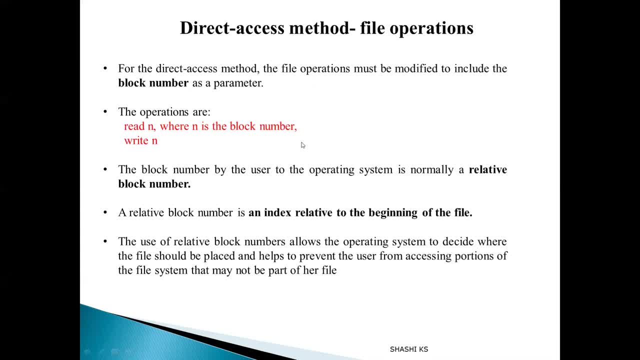 but here we have to randomly access any particular block number, so the user has to specify the block number also. so here commands will look like this: read n and write n where n stands for your block number. but the block number which is mentioned by the user is only a relative block number. it is not the actual block. 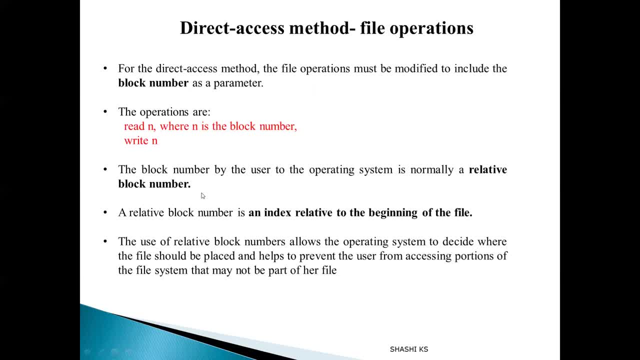 number. why? why the relative block numbers are provided by the user, is it? it helps the operating system to prevent the user from accessing some undefined, from accessing those portions of the file system which the user is not allowed to access. so, this relative block number given by the user, there will be an index. 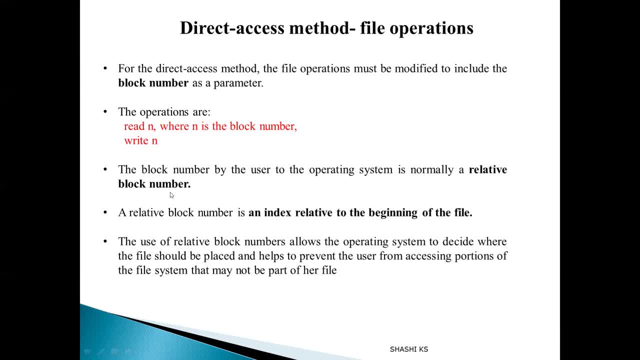 related to the beginning of the file, for example, if the user may specify a related block number like 0, which which might be actually in some disk address like 14544, purely digital. so this mapping of the relative block number with the actual disk address will be done by the. 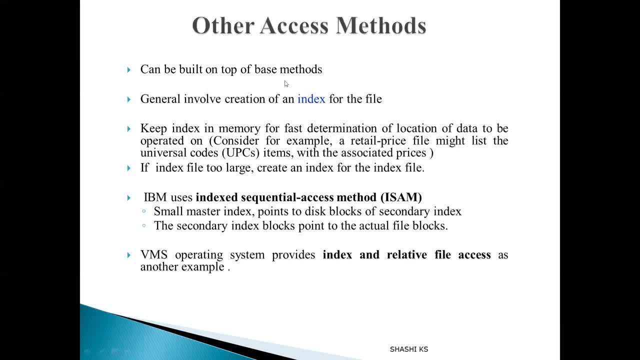 operating system. so you also have other type of access methods to check the entry of the disk, apart from sequential and direct access, and that is called indexed access method. so in index access method, index is like the index of your book. the index will contain pointers to the various blocks. 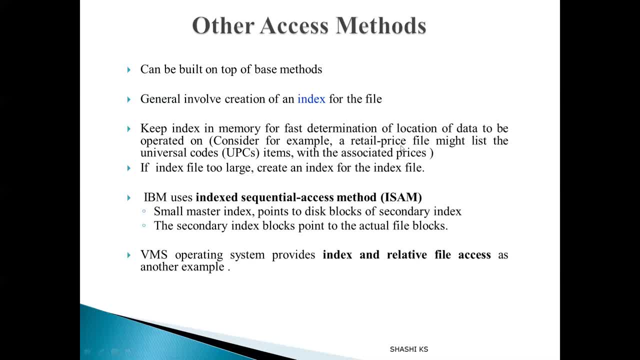 okay, let's say, for example, you have, you have a retail price file, and this retail retail price file maintains the product codes of various items as well as their prices. so this index may contain the first, it may contain the product code of the first record for that particular. 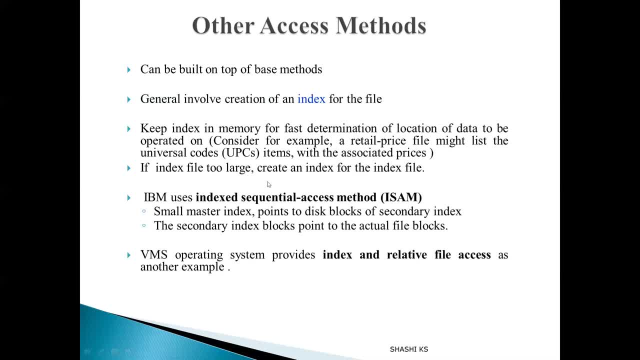 for that particular block. so in case, sometimes, if the disk, if the file system contains too much of files, then the index file also may be too large. in that case we can split the index file into two: master index and secondary index. and master index might be residing in the memory and the 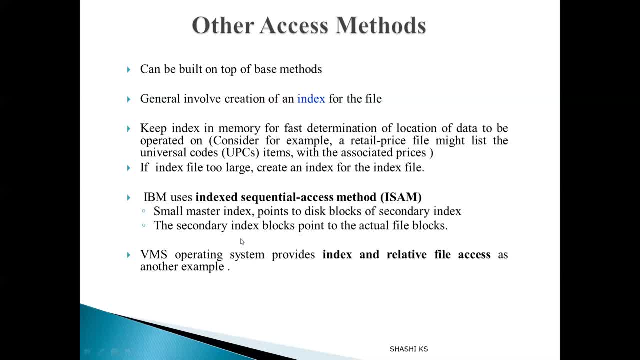 secondary index may be residing in the secondary storage device and it may actually point to the actual file blocks. okay, so this implementation in real time, ibm makes use of indexed sequential access method and vms operating system makes use of indexed relative file access method. so what is indexed sequential access method? we know that sequential. 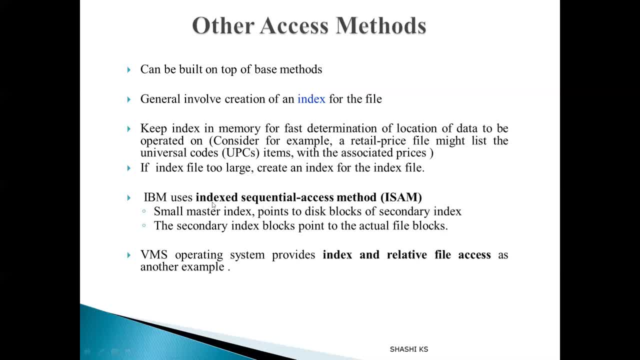 access means ordered access. index means we are waiting, maintaining some index which is going to be a pointer which is, uh, we are going to construct an index for the file. with the help of this index, which is going to contain pointers to the various blocks or the various records contained in your 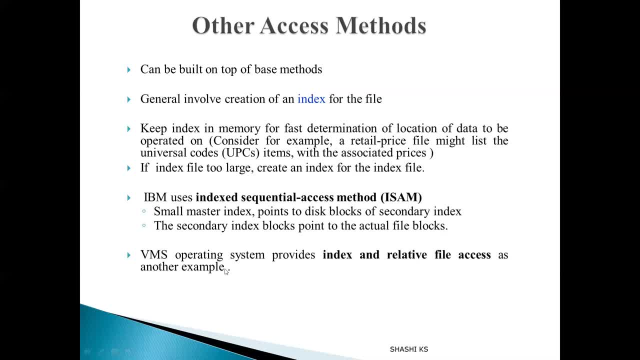 actual files. so ibm makes use of this method and vms operating system uses index with relative access. relative access means we know that it allows for random access to all those records on the random disk blocks. index is going to contain a pointer pointing to those actual disk. 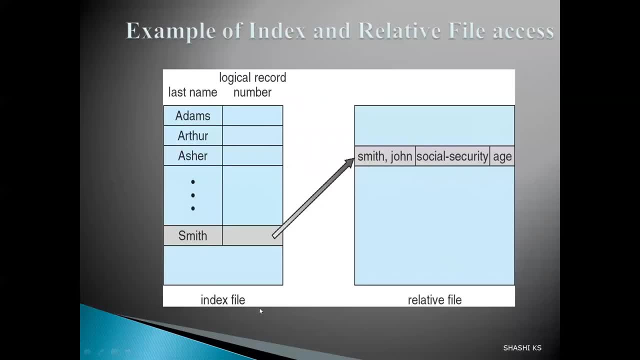 blocks. so index with relative access in vms operating system looks like this. so here you can see an index file. here you can see the actual file residing on the secondary memory which actually contains the last name, first name, social security number and the age of the employee. 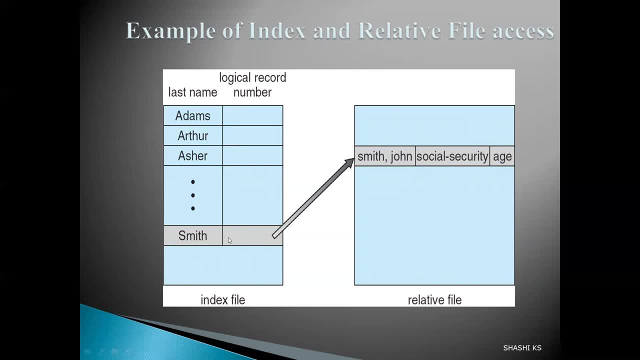 and the index file is being contains the last names of all the employees. actually it contains the last name. actually it contains pointer to the first record of each disk block. okay, so here you have the pointer where the first record's last name is smith, and this pointer points to the 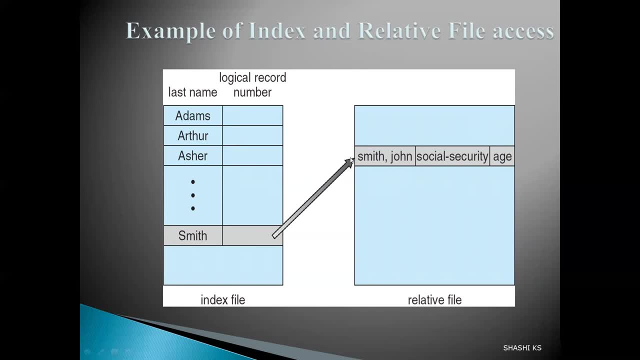 actual disk block or to the location of the actual disk block in the secondary memory. so in this way, index for index file is helpful for us to uh, it is helpful for us to make the search operation quicker. so instead of, whenever you want to search a larger file, instead of searching, 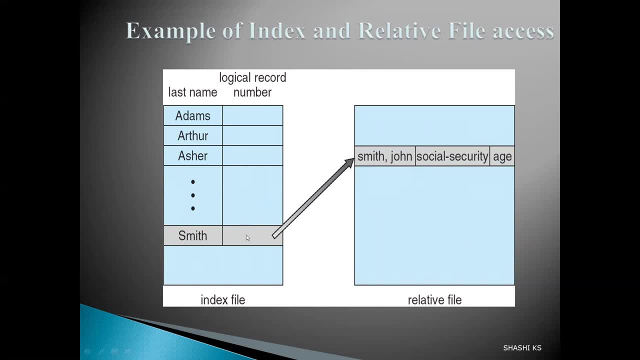 through the entire file for that particular record index is like the index of a book, which will actually contain pointer to the actual block containing your desired refer. so that is all about index and relative file access. 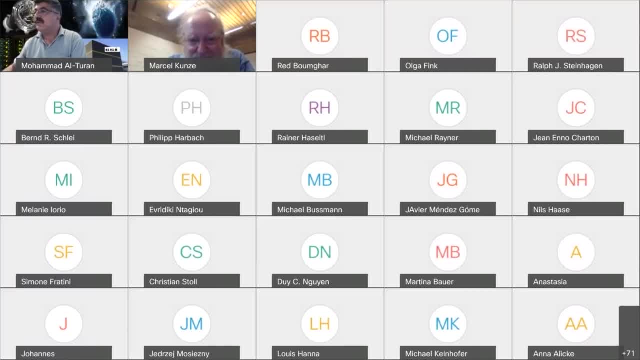 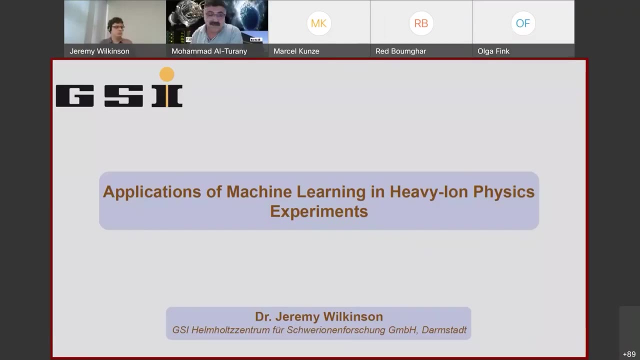 Now we move to the next talk. We stay in the physics and the particle physics, and now we have Jeremy. Are you there, Jeremy? Hello, Hello. I will speak to us also further about the tracking and about the high energy physics experiment. So Jeremy graduated from university in high energy physics. 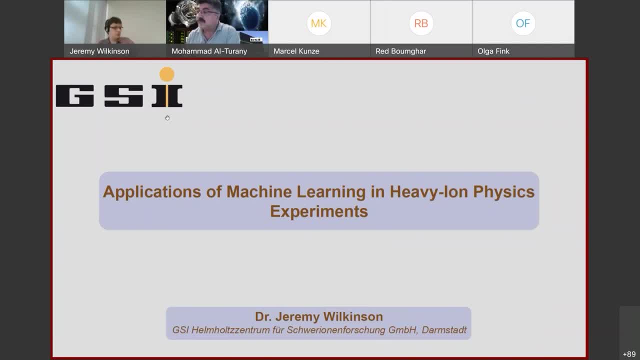 And at that time he worked for the ALICE collaboration, one of the four large experiments at CERN. He was also as a fellowship in the ENFN in the University of Polonia, also in the ALICE collaboration, And since last year he joined us here at the GSI working with machine learning, applying machine learning technique for track reconstruction for the study of ray signals in the ALICE experiment and in the physics analysis. 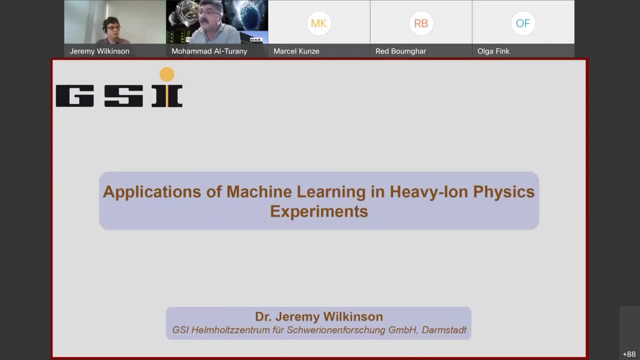 And Jeremy. Jeremy will speak to us about applying machine learning analysis technique to particle physics. Go ahead, Jeremy. Okay, yeah, thanks very much for the introduction and thank you for the invitation as well. It's my great honor to give this talk about some of the ways in which we apply machine learning techniques in the experiments at GSI. 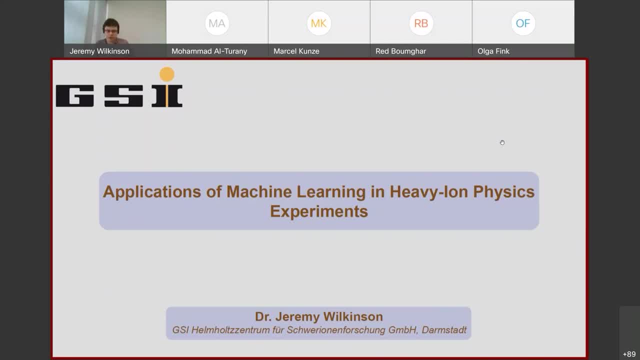 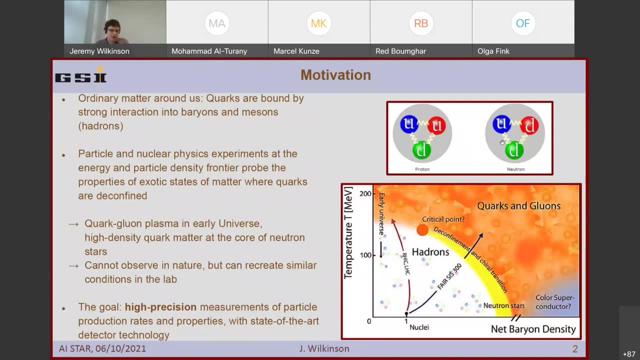 So, since I assume most of the audience isn't from a particle physics background, I want to start by just briefly outlining what it is we're measuring And why So. generally speaking, in the ordinary matter around us, quarks are bound together by the strong interaction through a mechanism called confinement into baryons and mesons. 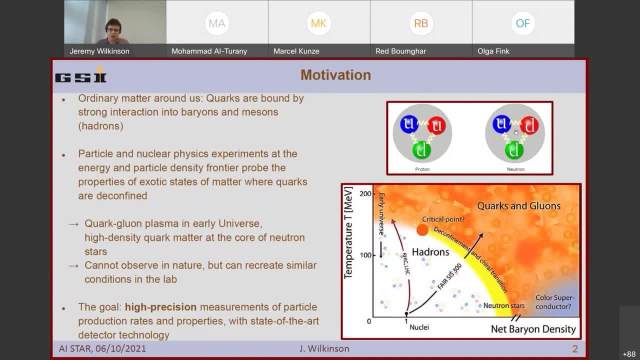 And the most common ones of these in ordinary matter are the proton and the neutron, which are two kinds of baryons, And what we want to do in particle and nuclear physics experiments is to probe exotic states of matter where these quarks are.